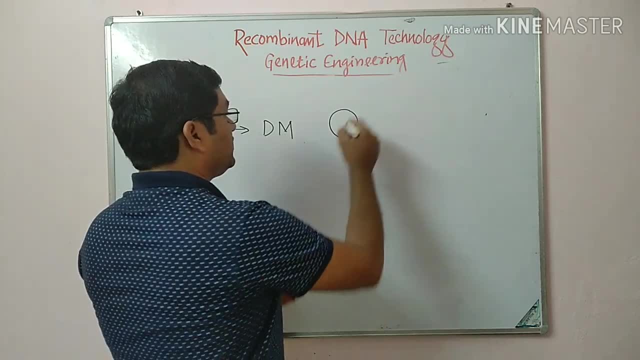 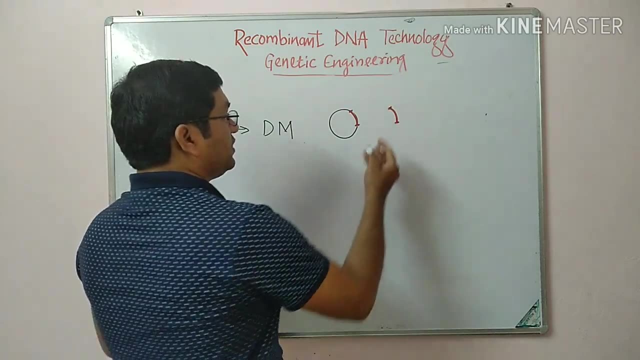 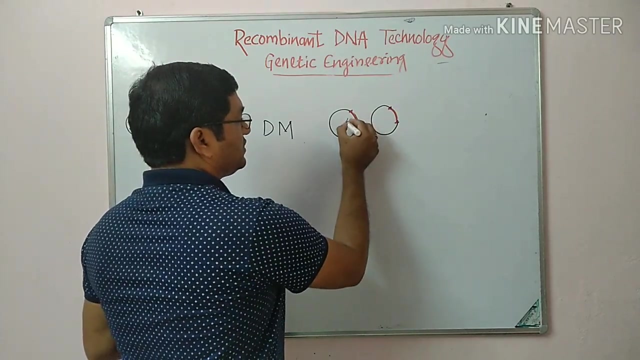 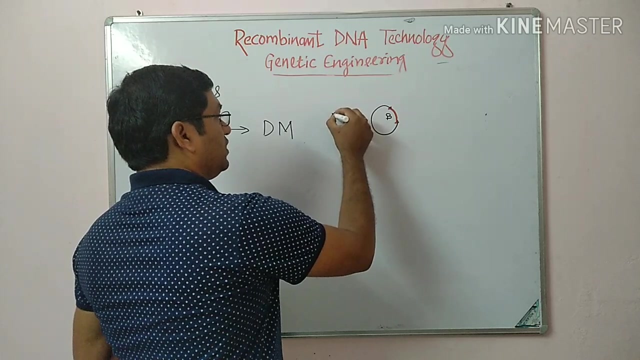 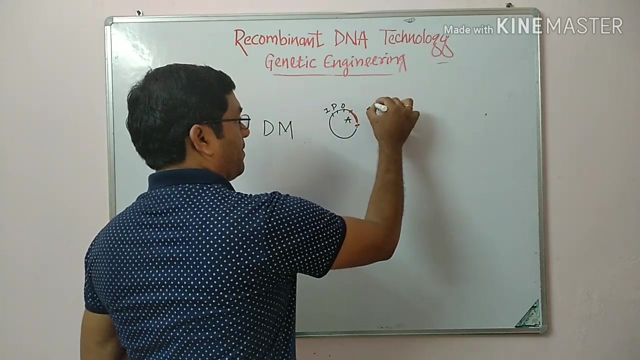 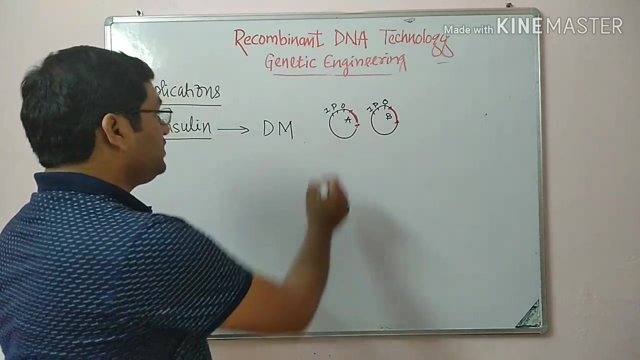 chain A is inserted and gene for chain B is inserted into a separate plasmid. This is a recombinant DNA with gene for chain A and gene for chain B, along with the lac operon concept, That is, IPO, And this recombinant plasmid, which contains gene for chain A and 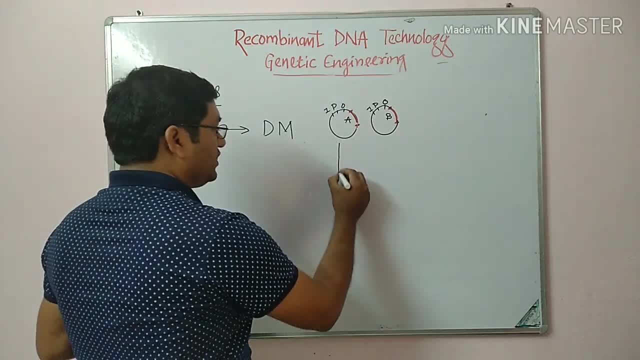 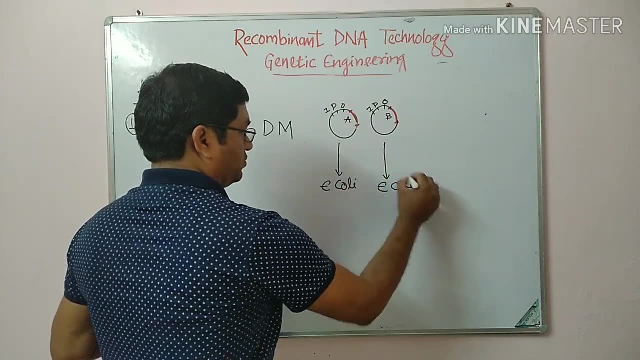 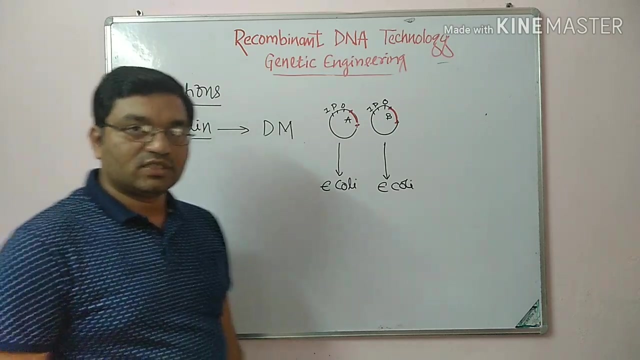 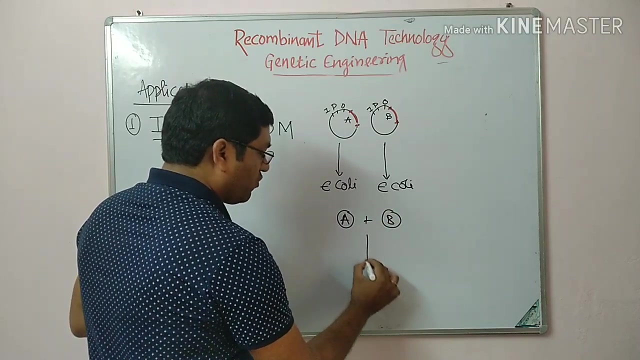 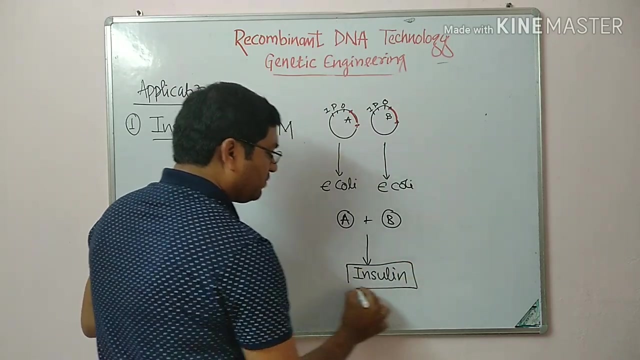 gene for chain B, they are introduced into a E coli. They are introduced into a E coli and after the isolation and purification, this chain A and chain B combine to form an insulin which is used in the treatment of diabetes mellitus. 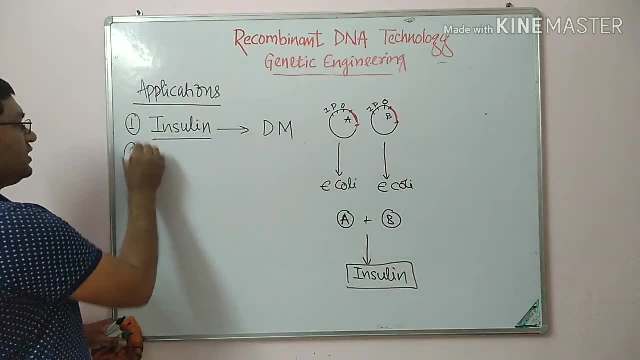 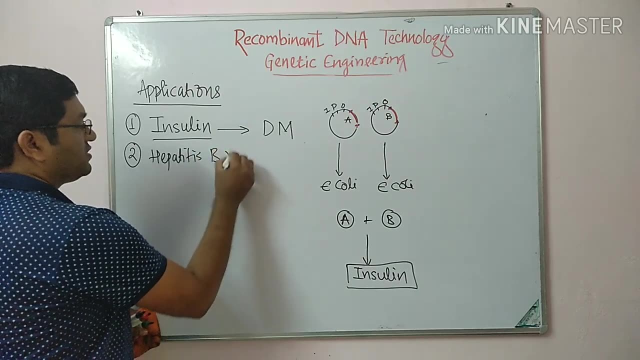 The second use of recombinant DNA technology is production of therapeutic drugs. This is the second part of recombinant DNA technology. It is the first and important use of recombinant DNA technology. The second important product of recombinant DNA technology is hepatitis B vaccine. It is 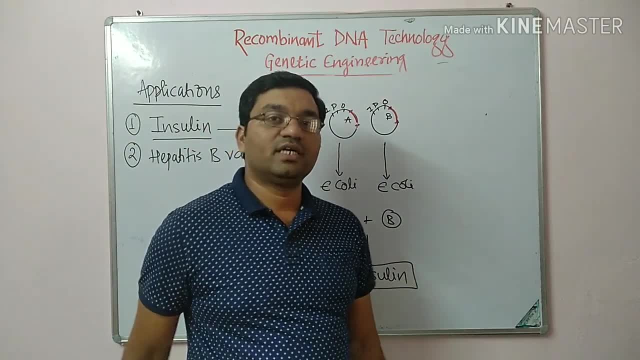 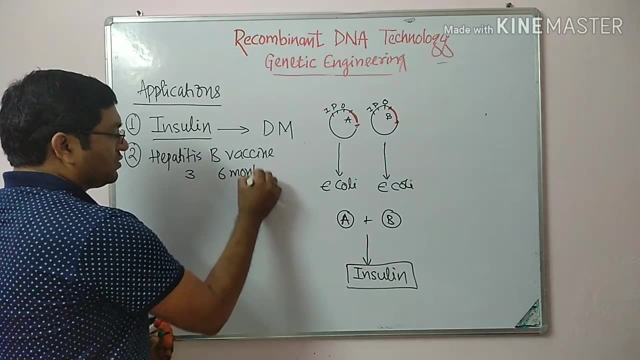 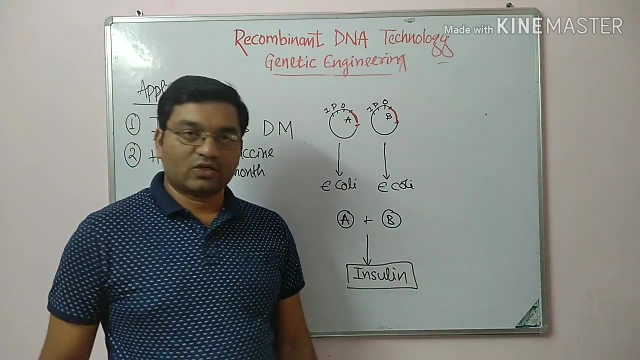 the first synthetic vaccine produced by the recombinant DNA technology. Three doses are required in an interval of six months. It is recommended for healthcare workers. It is produced by recombinant DNA technology. Thank you, Okay. The third one is the DNA vaccine. 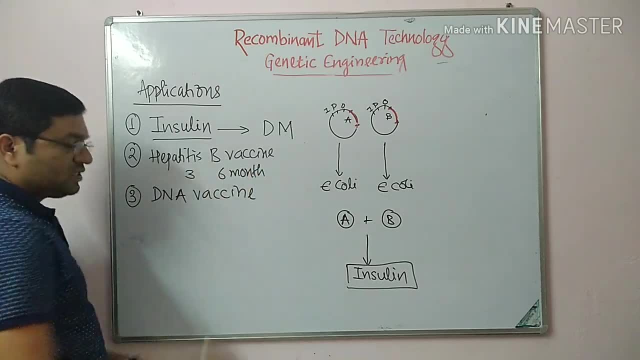 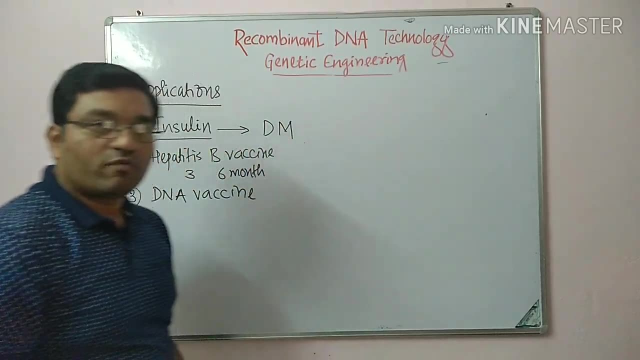 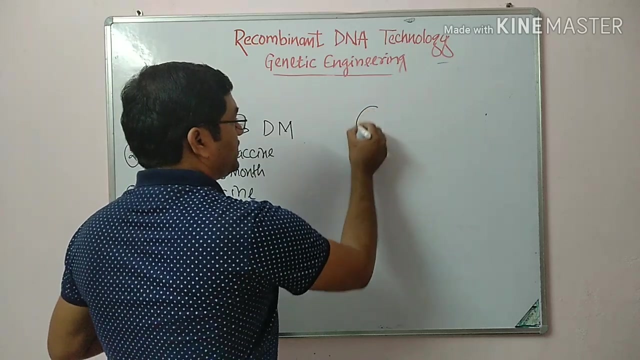 sangatairsihay một creekidente matavez. denk dat me능? DNA vaccine: This is the concept in which a plasmid with gene for particular antigen is inserted into a cell. Suppose this is a plasmid and this is a gene for particular antigen. 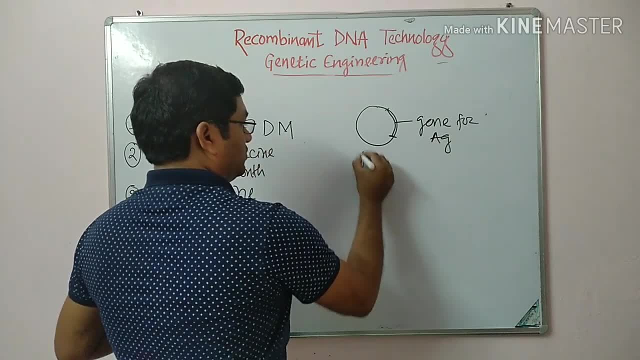 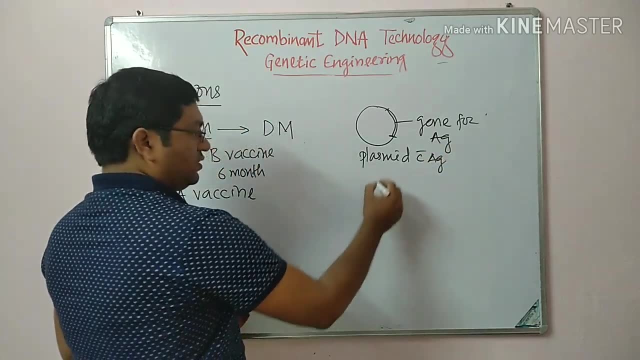 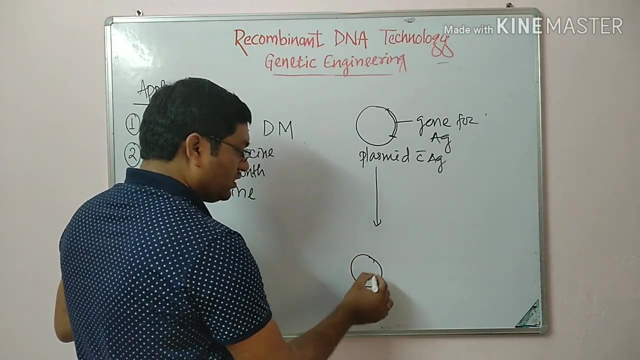 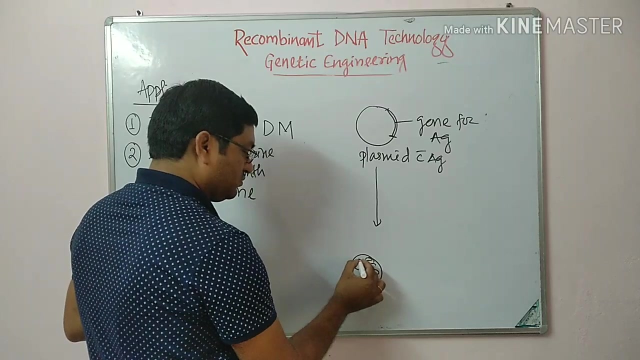 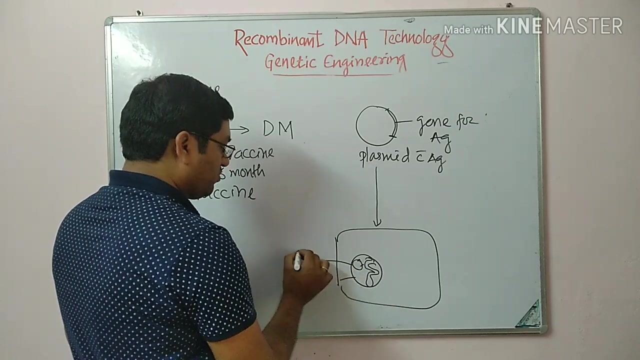 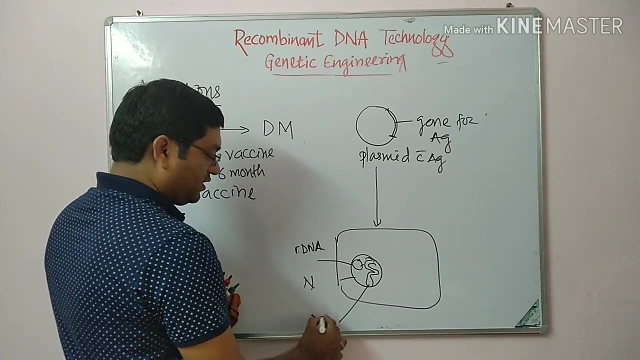 Agree, this is plasmid with antigen gene. it is inserted into a cell in cell. there is nucleus, in nucleus. this is a cellular dna and this is a plasmid with gene for antigen. this is a cell, this is nucleus. this is recombinant plasmid. this is cellular dna and this is a cell in this, by the process of 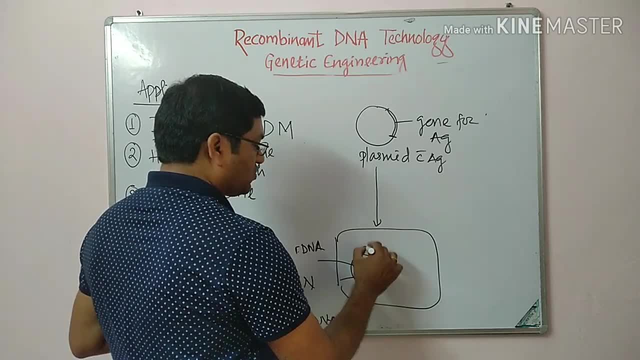 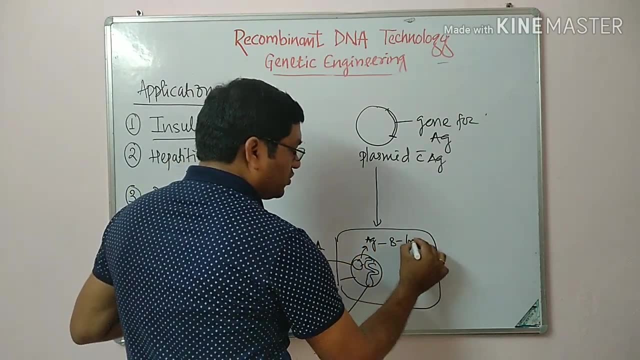 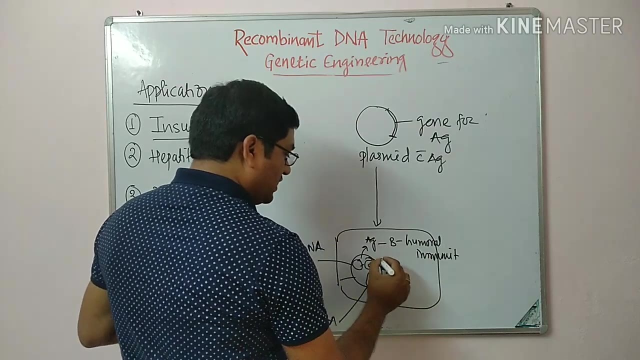 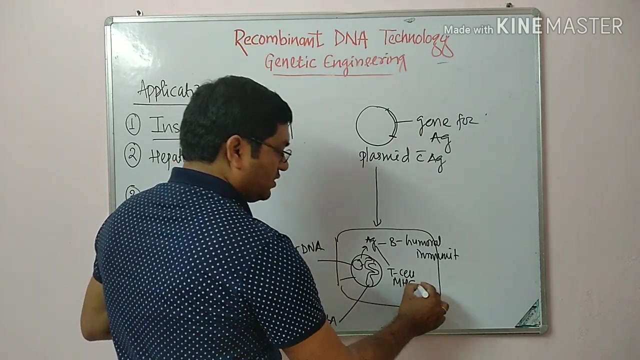 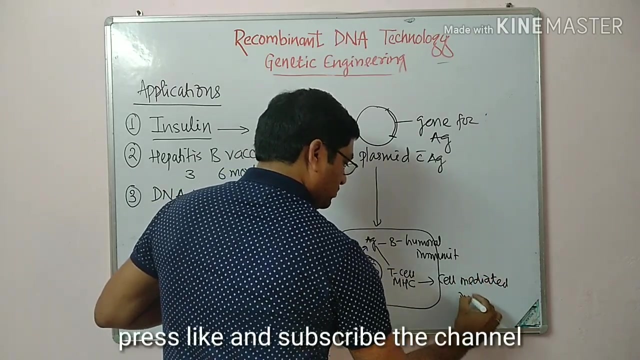 transcription and translation. there is synthesis of this antigen in the cell, which is, along with the b cell- it is responsible for the humoral immunity- and along with the t cell and mhc- t cell and mhc- it is responsible for cell mediated immunity. so this is a concept of dna vaccine. 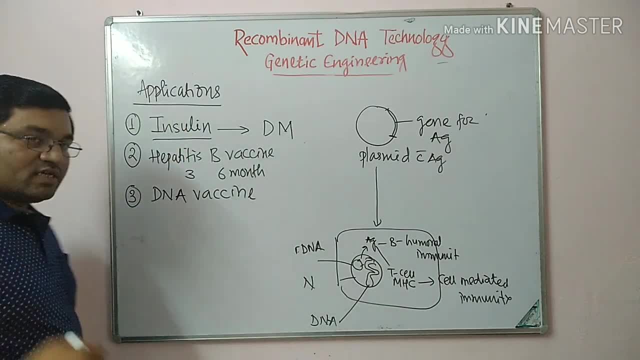 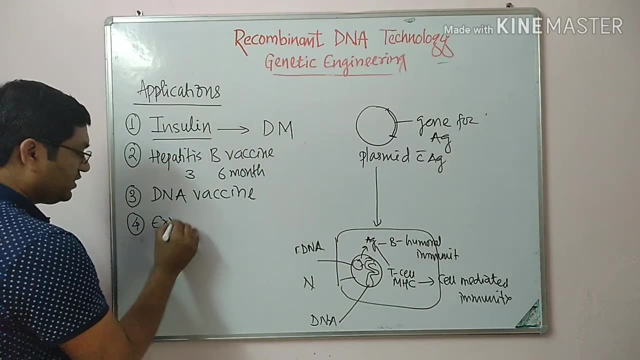 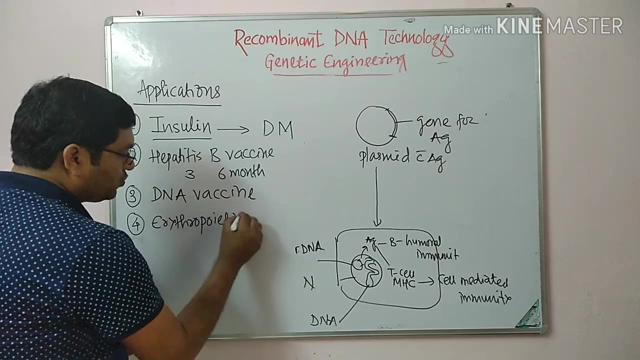 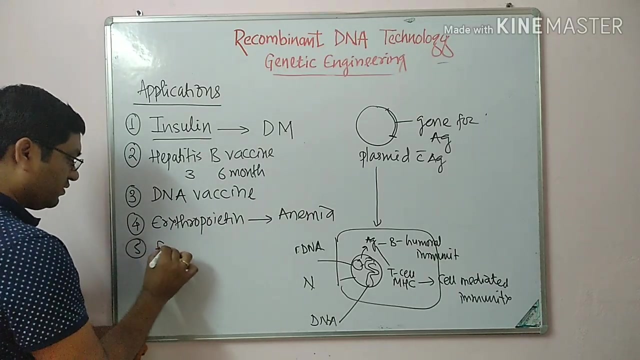 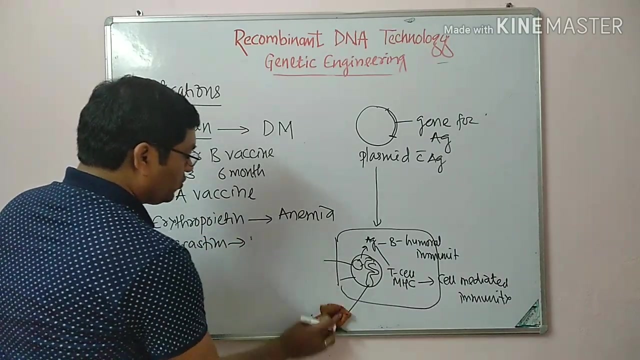 now there are various important products which are produced by the recombinant dna technology. the first four one is the erythropoietin. erythropoietin, which is used in the treatment of anemia. then fifth one is the philgrastim. it is used in the treatment of neutropenia. 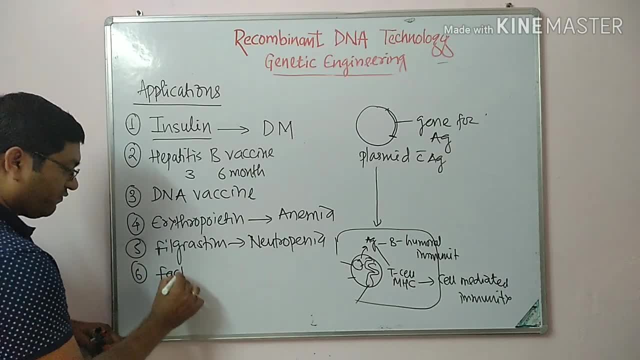 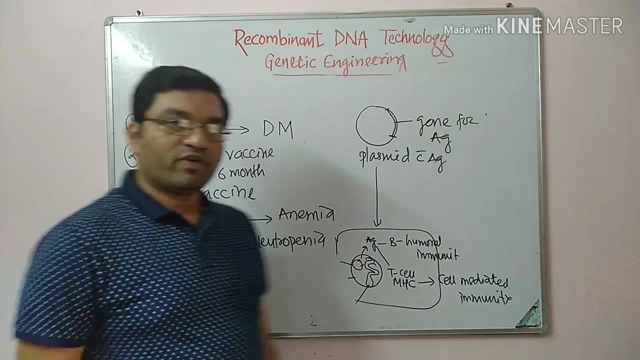 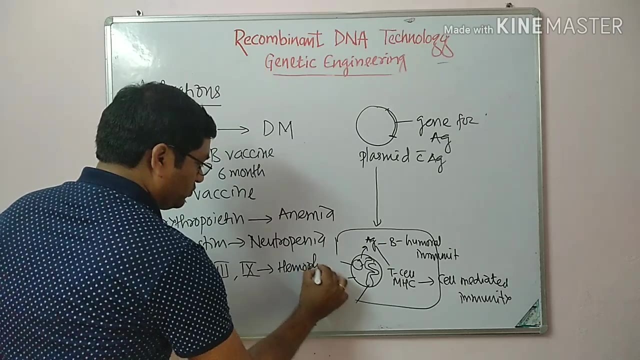 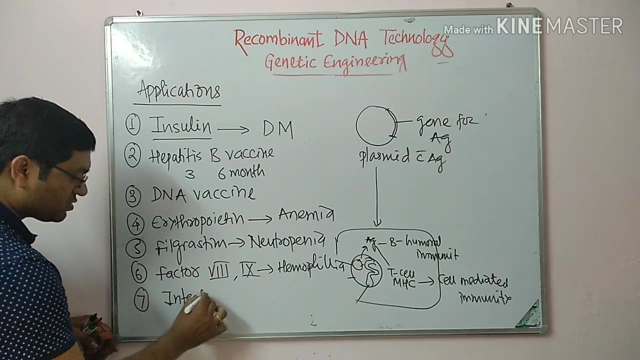 then coagulation factors, factor 8, factor 9, which is used in the treatment of hemophilia a and hemophilia b, so it is used in the treatment of hemophilia. then seven, it is used for the preparation of various interferons, which is used in the viral 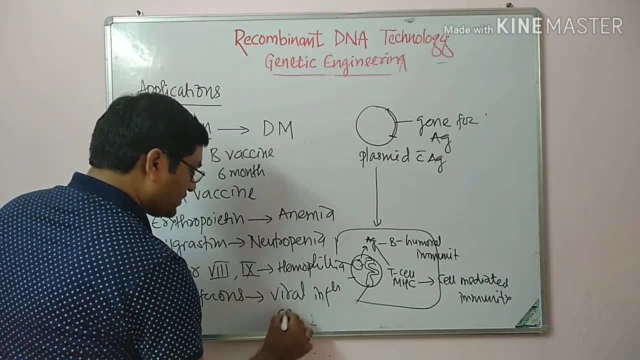 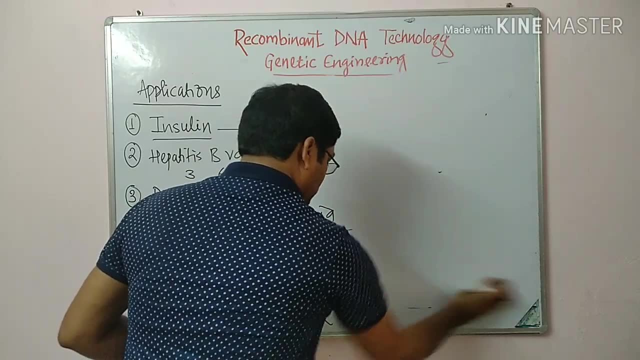 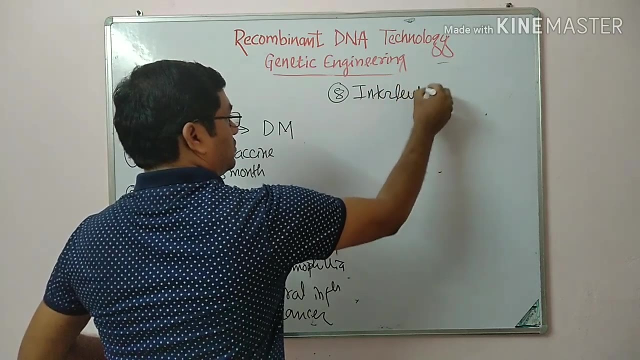 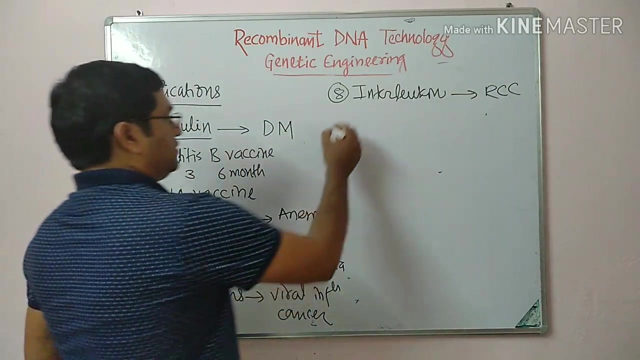 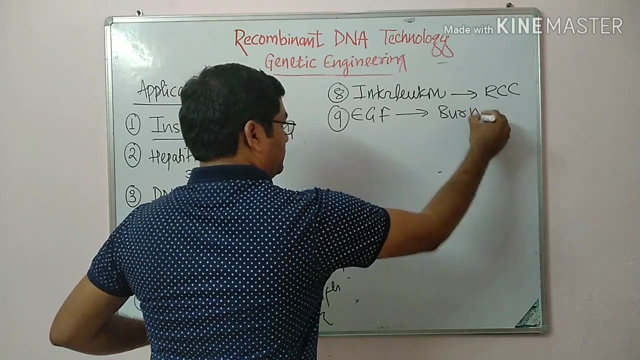 infection and various cancers and it is used in the production of interleukins. it is used in the production of interleukins which is used in the treatment of renal cell carcinoma. various growth factors, epidermal growth factor which is used in the burn, and l je двух. 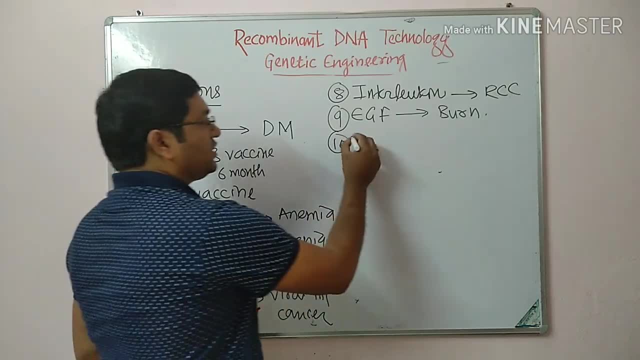 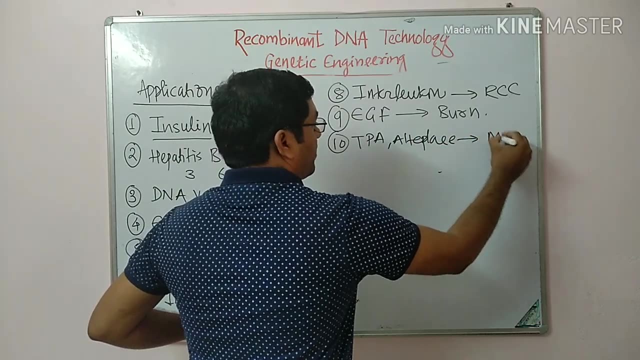 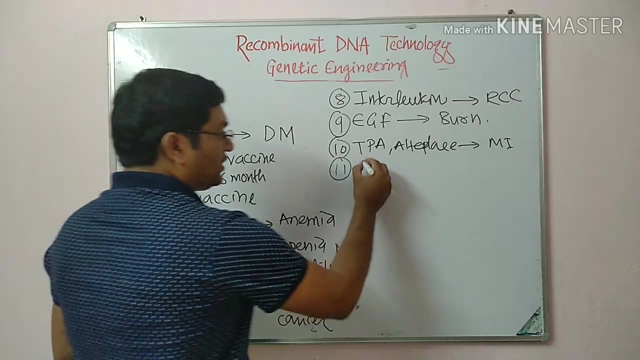 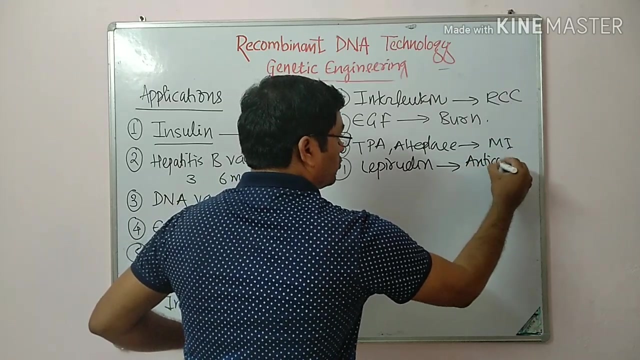 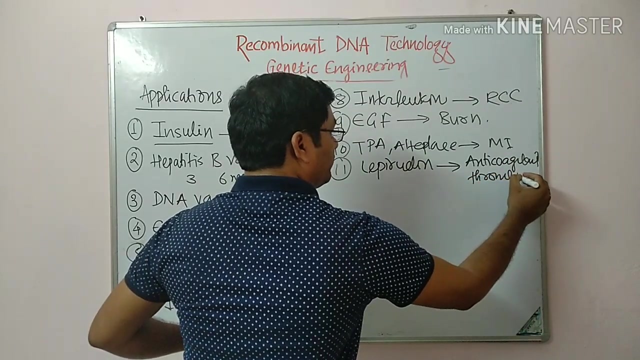 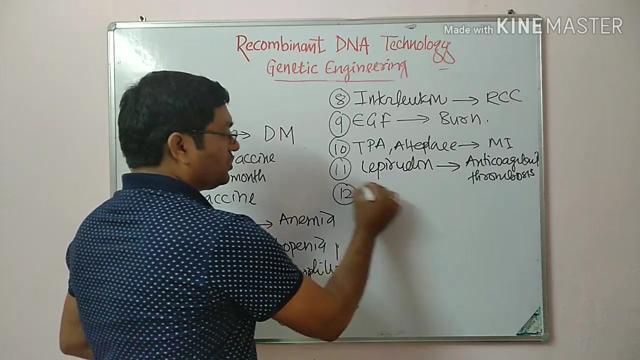 hymen, addition of the my award uj dna treatment Forces of dna also, and also there is theraptic, so the so here in thrombosis. so these are the different products which are given by the recombinant dna technology. it also gives hormone, that is fsh, which is used in infertility. 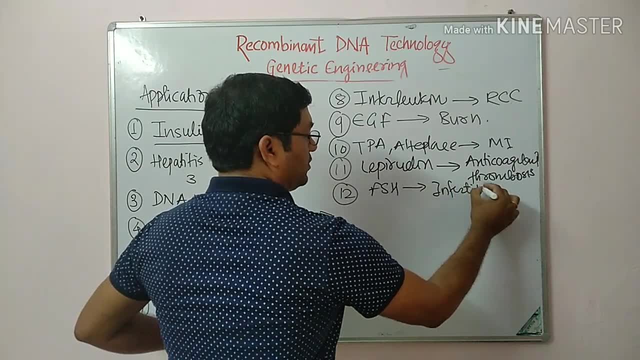 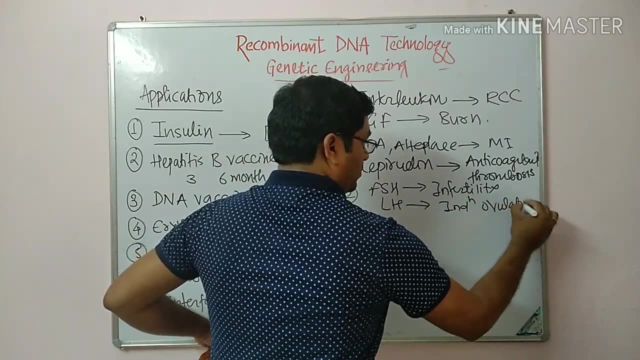 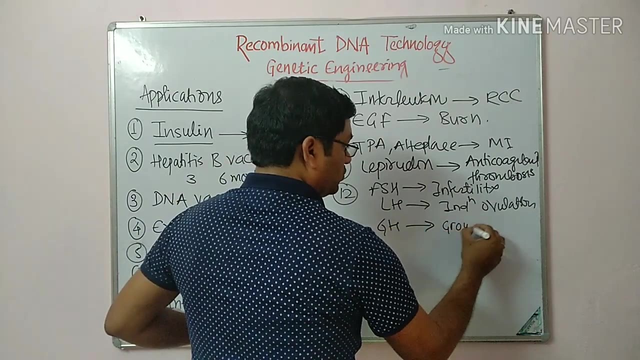 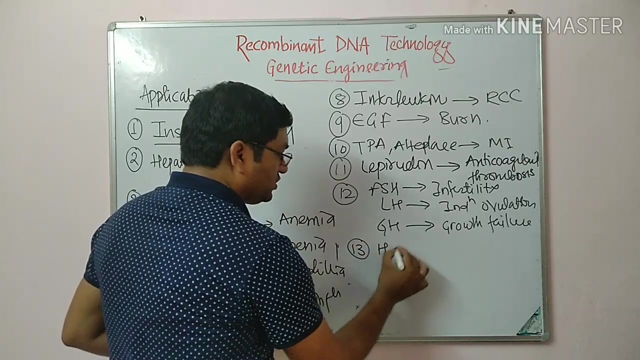 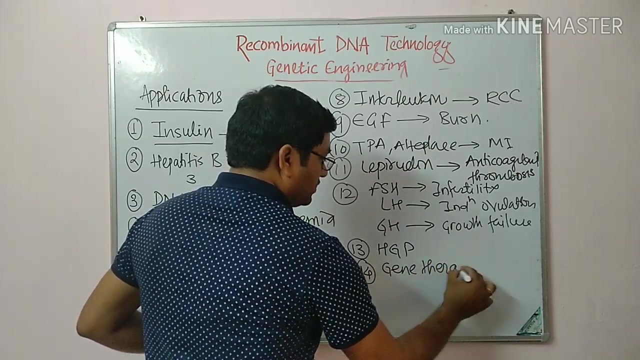 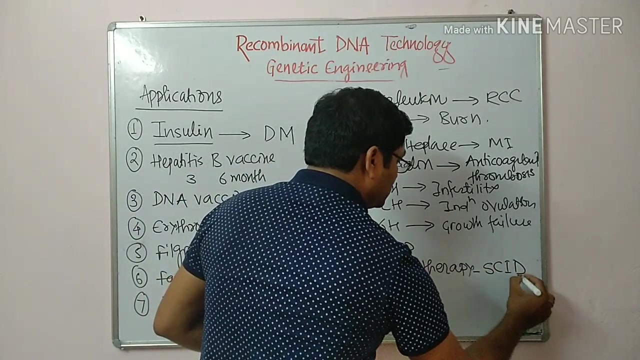 infer infertility. then lh, which is used for induction of ovulation and growth hormone. it is used for growth retardation, growth failure. again it is utilized in the human genome project, then in the gene therapy for correcting various diseases. this gene therapy was tried on severe combined immunodeficiency. 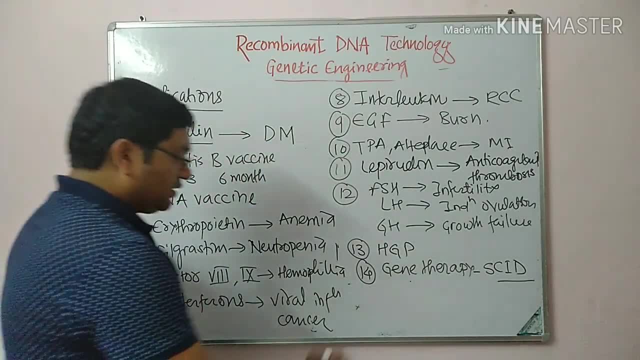 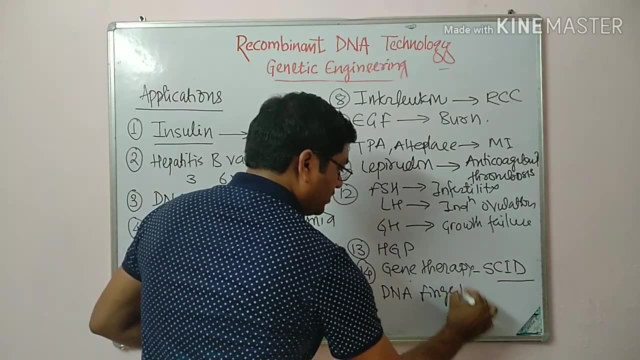 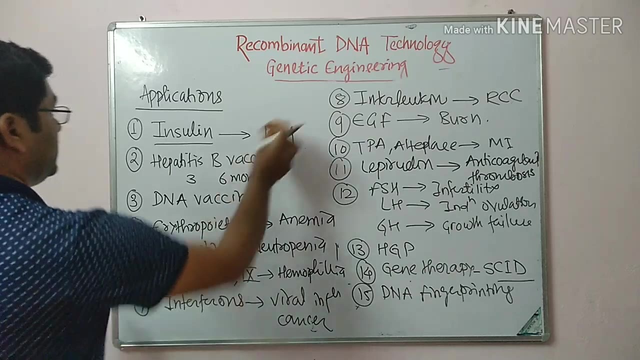 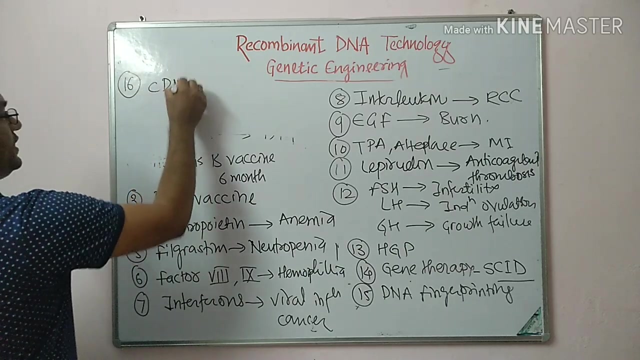 syndrome, and it was used in the human genome project, then in the gene therapy for correcting syndrome for the first time. then again, it is utilized in the dna finger printing. dna finger printing for identification of criminal thieves and rapists. then next one is the. it is used for construction of complementary dna library.